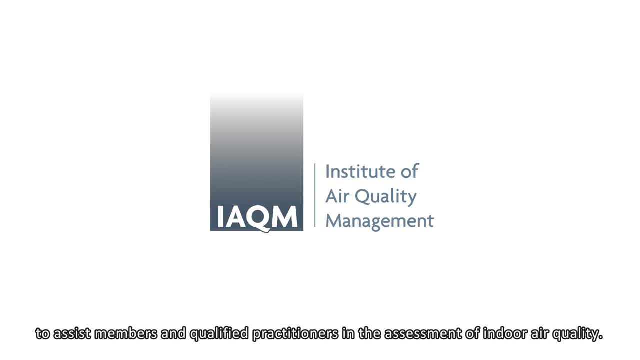 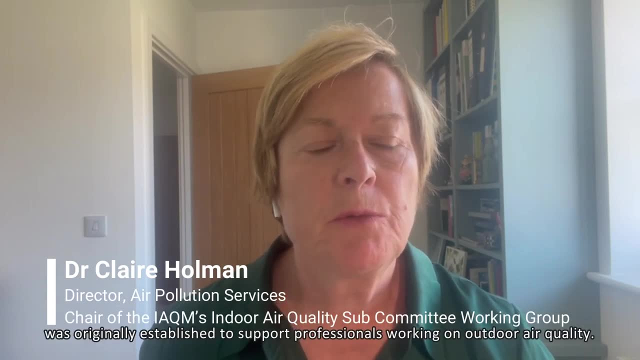 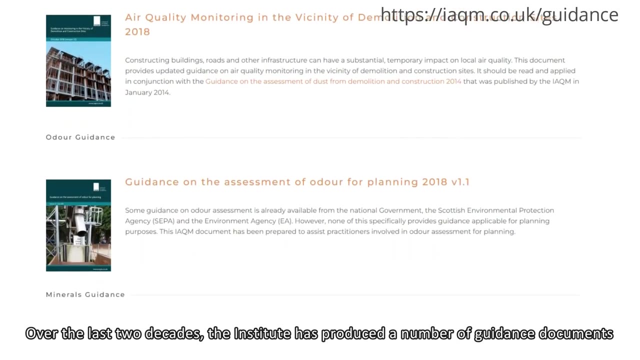 to assist its members and qualified practitioners in the assessment of indoor air quality. The Institute of Air Quality Management was originally established to support professionals working on outdoor air quality. Over the last two decades, the Institute has produced a number of guidance documents to assist our members and others in their work. 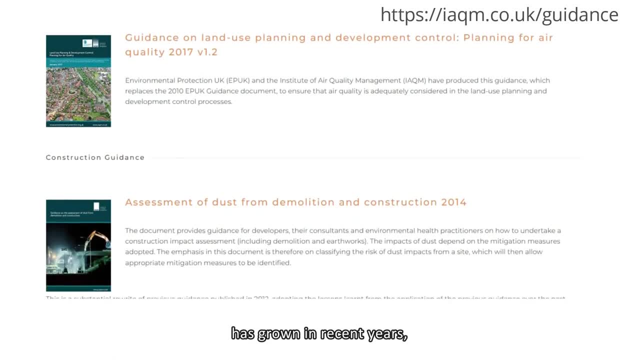 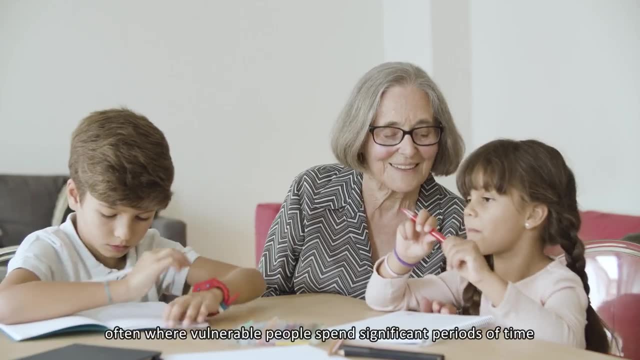 Interest in indoor air quality has grown in recent years and there was the realisation that there are many indoor environments, often where vulnerable people spend significant periods of time, where exposure to indoor air quality is limited. Exposure to indoor air pollution was simply never considered. 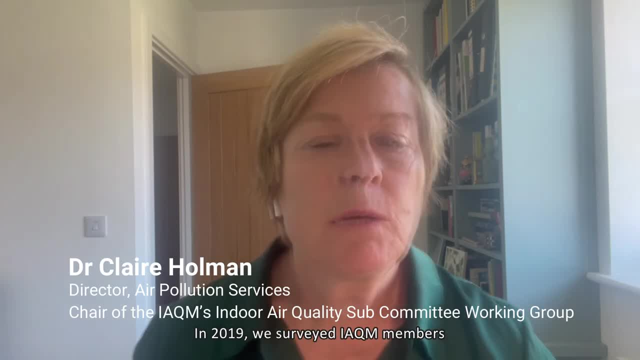 In 2019, we surveyed IAQA members to see if there was any appetite to broaden the remit of the Institute. Over 80% agree the Institute should include indoor air quality And in early 2020, a group of interested members started producing guidance on the assessment of indoor air quality. 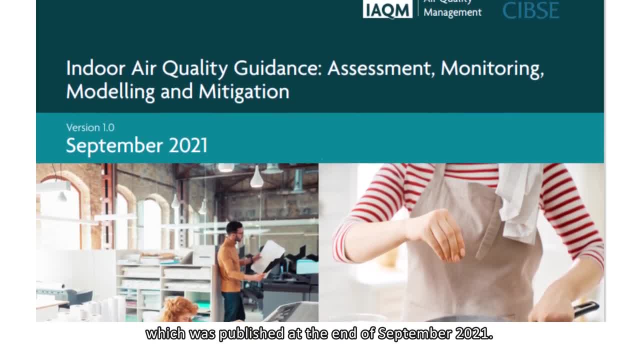 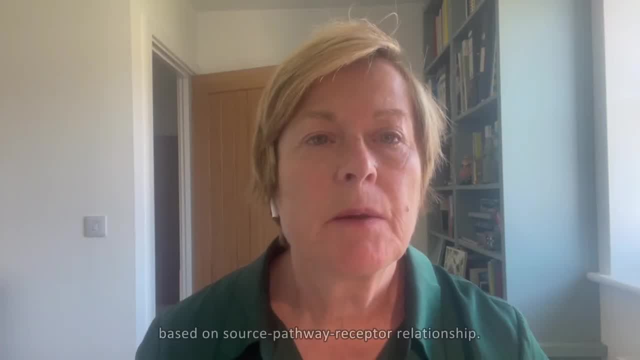 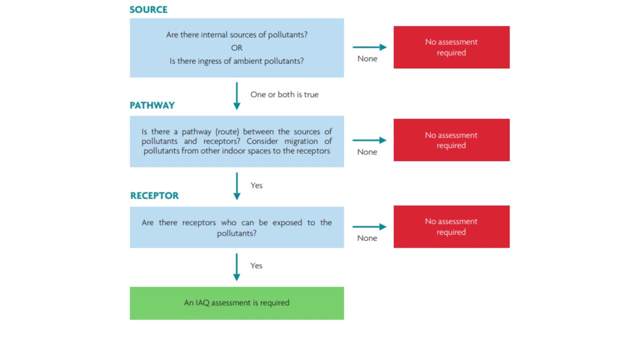 which was published at the end of September 2021.. Thank you. Let's have a look at the guidance. The guidance describes a risk-based assessment method based on the source-pathway-receptor relationship. It takes account of the lightning magnitude of different pollution sources. 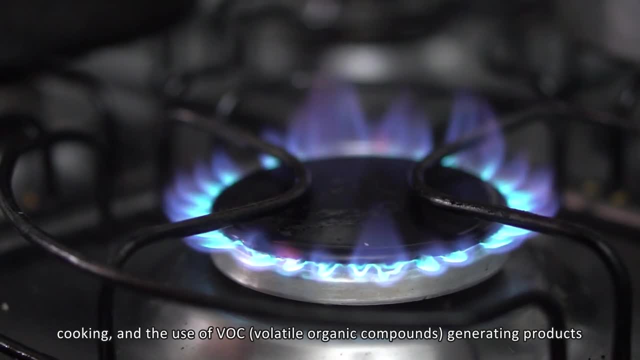 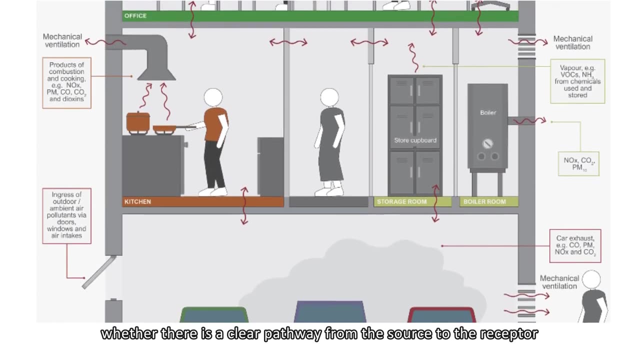 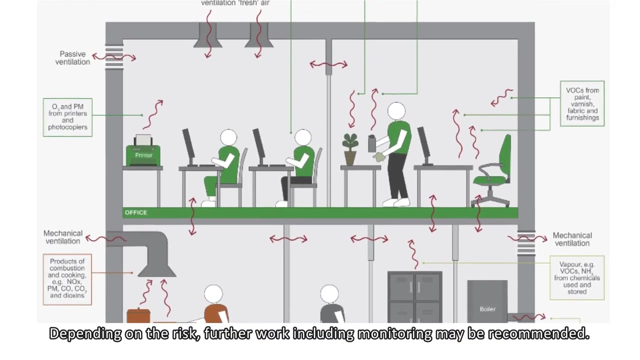 such as the ingress of outdoor air cooking and the use of VOC-generating products, whether there is a clear pathway from the source to the receptor, and the duration of exposure, Depending on the risk. further work, including monitoring, may be recommended. 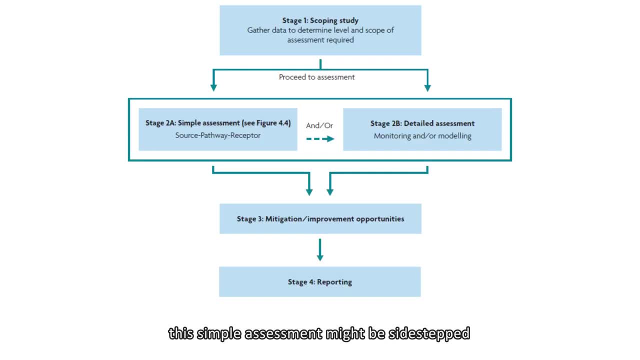 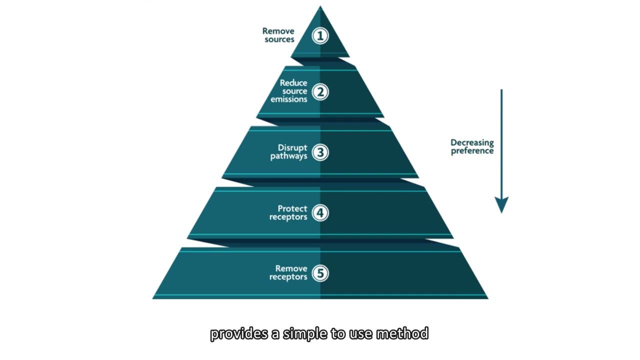 If there is a known high risk, this simple assessment might be sidestepped with appropriate monitoring and or modelling undertaken, depending on the nature of the indoor environment being investigated. The IAQM guidance provides a simple-to-use method for identifying where there may be a high risk from indoor air pollution. 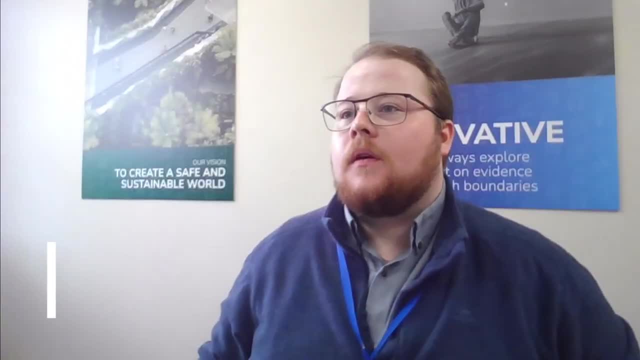 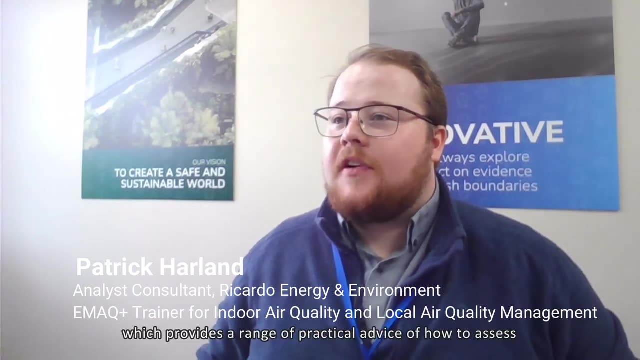 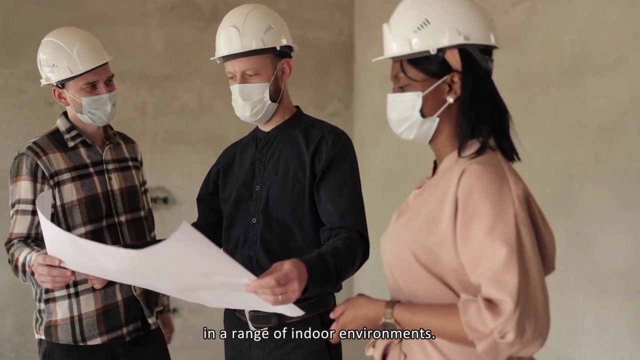 with recommendations on further actions to take. I am an air quality professional and I find the IAQM Indoor Air Quality Guidance to be a comprehensive guide which provides a range of practical advice on how to assess, monitor, model and mitigate indoor air quality in a range of indoor environments.